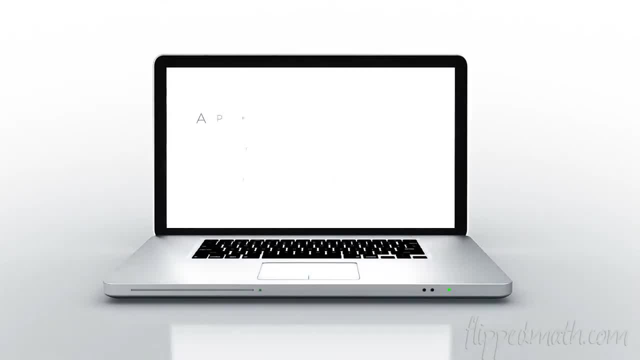 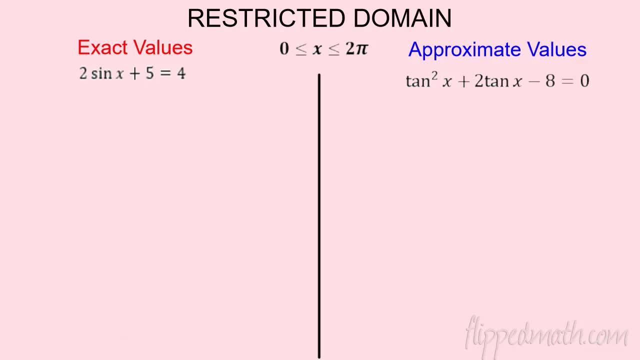 All right, here we go. Let's take a look at the next section. This is Mr Bruss. In this section, we're going to combine your two favorite things: trigonometry and solving equations. It's going to be awesome. Let's get in there and get started. Let's solve this equation. 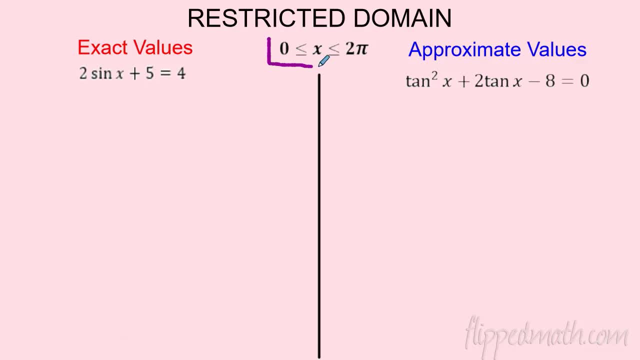 over here Notice, we're going to start off by restricting the domain. So we're going to say I'm only talking about answers between 0 and 2 pi, because there's so many different trig values there. So we're going to limit it for these first couple examples, When I say exact. 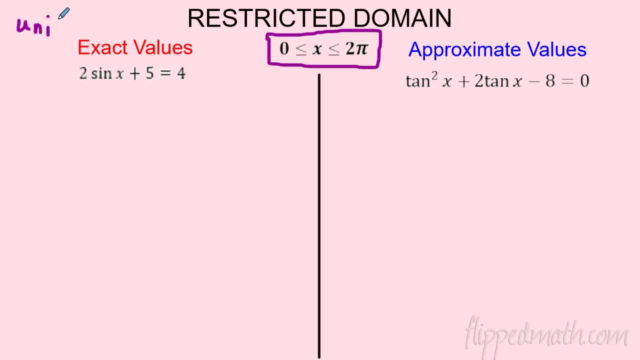 values. that means hey, yeah, use the unit circle, Check that out. I want the exact special case where that happens. So use the unit circle over here. When we say the approximate values, that's where we're going to type them in the calculator. I guess you could go old school. 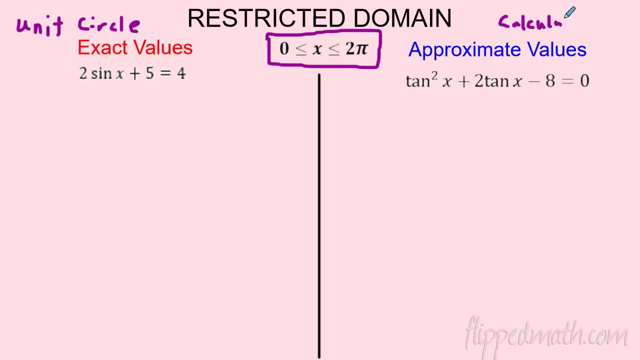 and find a table that generates them, but that would be ridiculous. Just use the calculator and find these approximate values over here. All right, let's solve this bad boy here. So, just like any equation, I want to get x by itself. So I'm going to start working. 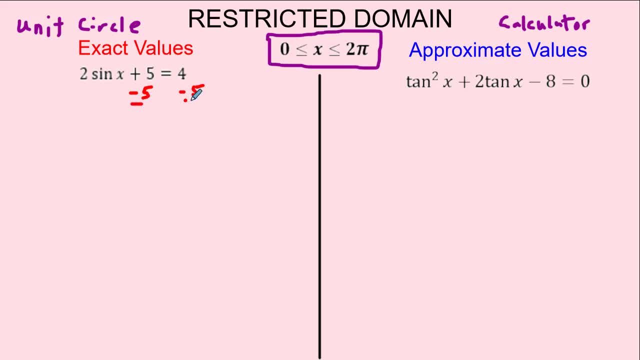 backwards here and say, okay, let's subtract 5 from both sides, So it's just like a normal equation. Boom, those cancel out. We're looking at what 2 sine x equals negative 1. Awesome, And then what are we going to do here? Yeah, just divide both sides by 2.. So we're getting that. 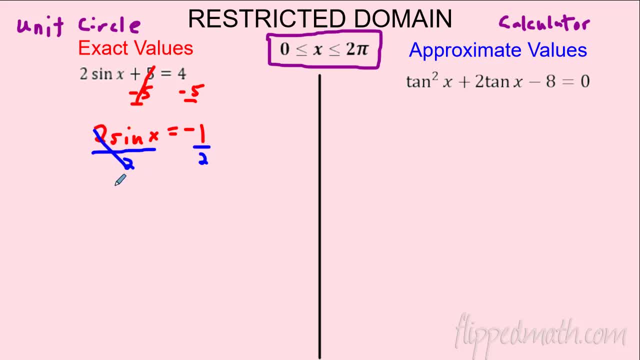 trig function by itself. Boom, there it is. And now we're looking at: hey, the sine of x is going to equal negative 1, half Awesome, All right. so when we're here, what do we got to do to get x by itself? We're going to take the. 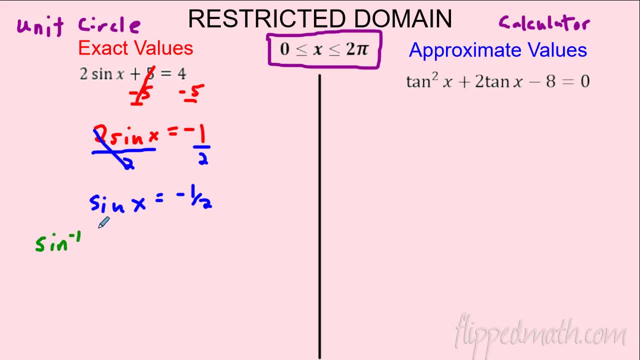 inverse sine of sine. So to cancel out like square cancels, the square root, we're going to inverse sine the sine of x. Whatever you do to one side, you got to do the other side. So we're going to come over here and take the inverse sine of what Negative 1 half If you want to use arc. 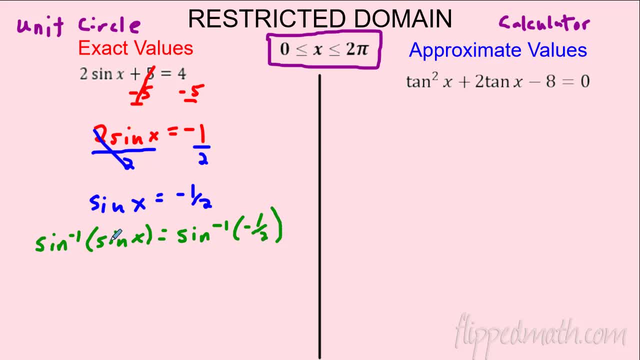 sine. totally legit. You can use that. What's the goal here? So these cancel each other out. That was our whole goal and we're left with plain old x. And now we got to think about: hey, what is the inverse sine of negative 1 half? So we got to think: 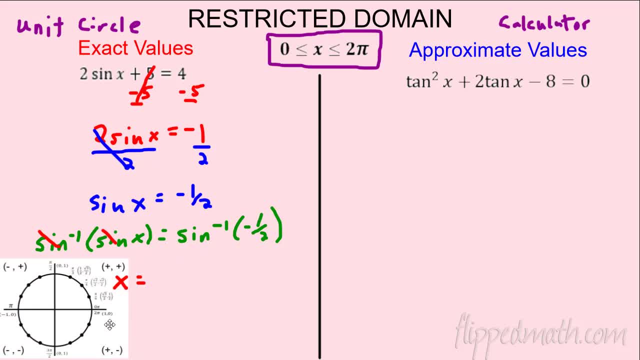 about our old unit circle there. Let's bring that bad boy over here. And where in the world does it equal negative 1 half? So the sine value is the y. We're going to look at what It's going to be some. 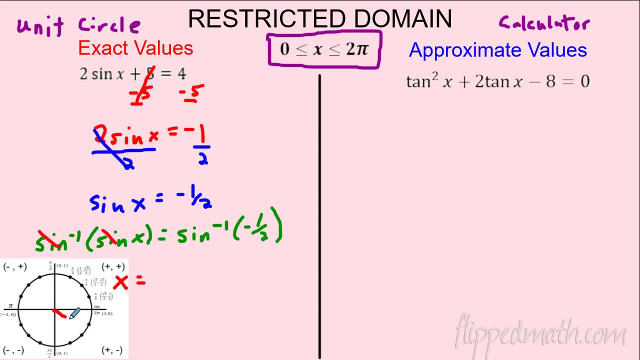 kind of thing of pi over 6, but it's negative, So it's going to be down here, It's going to be this bad boy here, this bad boy here. So we're talking about what? Pi over 6, after pi. So I know. 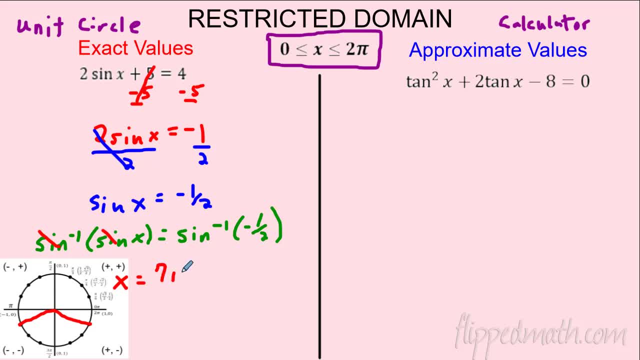 6pi over 6.. 6 is pi. So add one more. I'm at 7pi over 6.. And where else can it happen? This bad boy over here? He's not quite 12pi over 6, which is 2pi. So he's one less. He's 11pi over 6.. So there we go. So there are two. 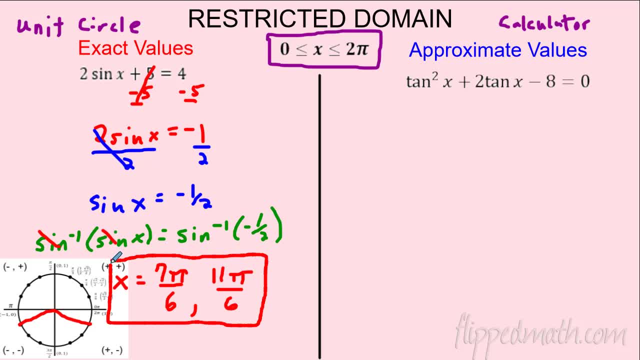 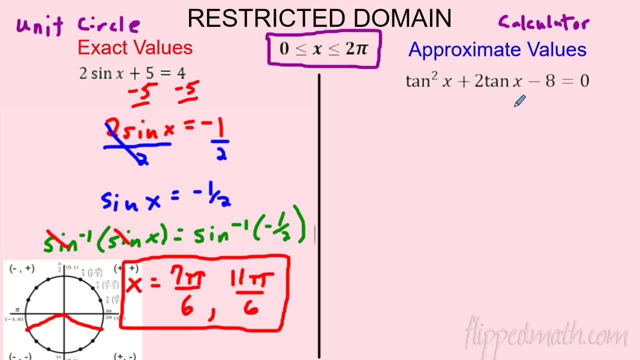 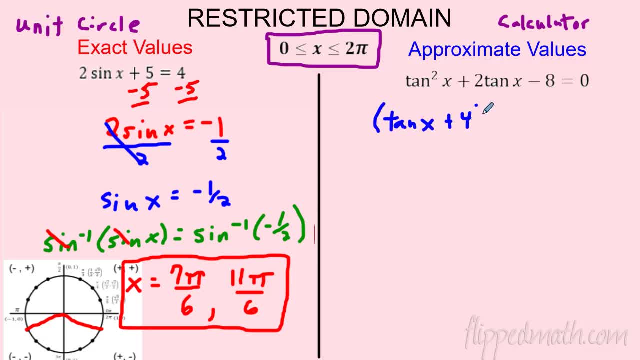 x plus 4, and we're going to times that by the tangent of x minus 2, because what multiplies the negative 8 and adds to 2, it's going to be 4 and 2. so we're just putting a little trig in there. 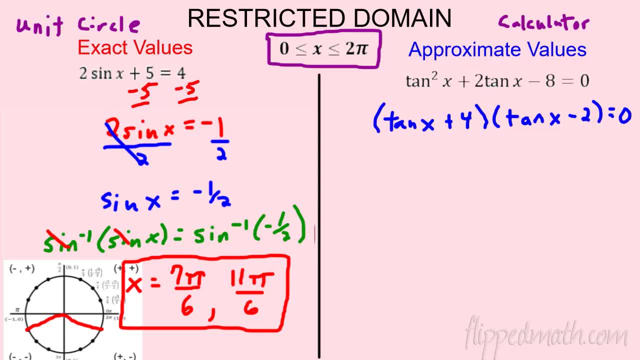 get a little triggy with it. awesome. now, when we have it this far, what are we going to do? we kind of look at both parentheses separately. we're going to say, okay, when does the tangent of x plus 4 equals 0? that's going to make one answer. that's a little zero product rule where anything times. 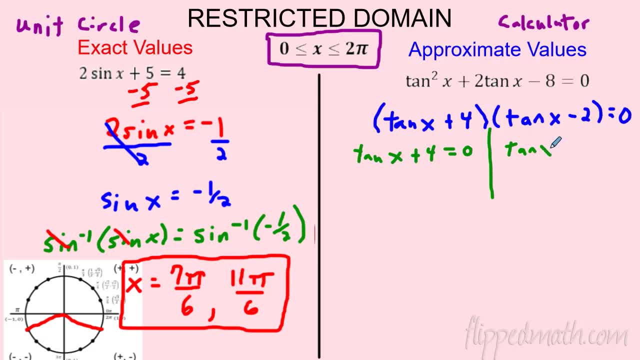 0 is 0. what makes this parentheses? well, if tangent of x minus 2 equals 0. so if either one of these equals 0, 0 times anything is 0, we get an answer. so solve this. I'm just going to bring the 4 over. 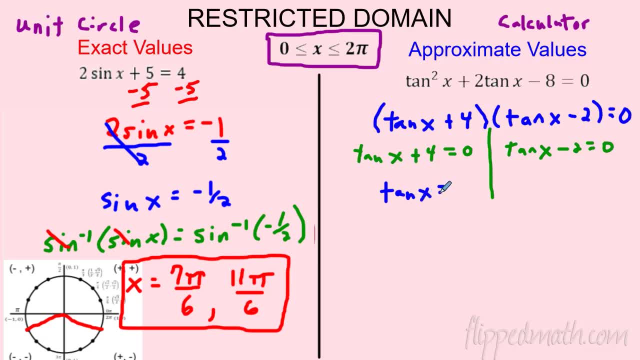 if that's cool. I'm not going to show that step. I think we're cool in that- subtract 4 from both sides. so we get: when does the tangent of x equal negative 4? add 2 to both sides on this one and we're going to say: when does the tangent of x equal 2? these are not on the unit surface, all right. 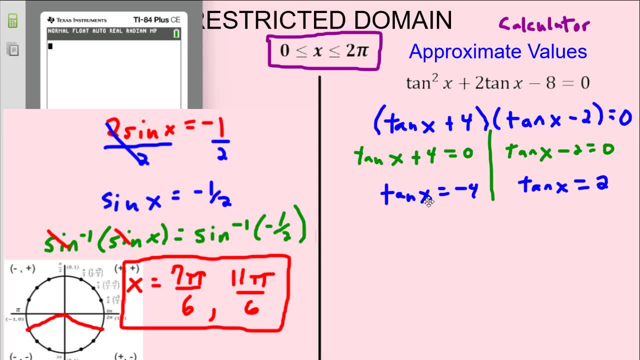 let's put these bad boys in the calculator and see what we come up with here. so I'm looking for: when does tangent equal 0? and we're going to say: when does the tangent of x equal 2? and we're going to say: when does the tangent of x equal negative 4? so we're going to invert inverse tangent that. 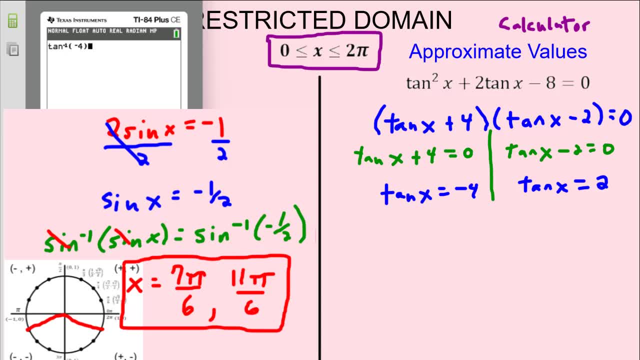 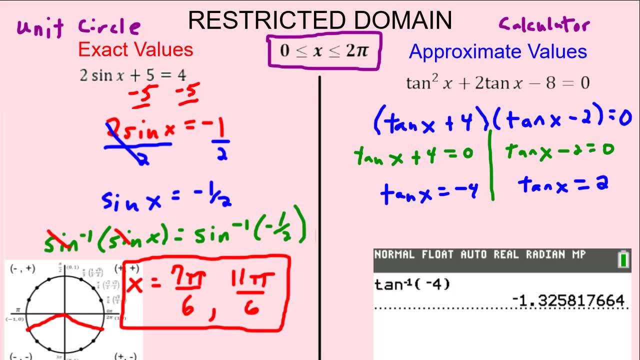 bad boy right there. so we're going to say inverse tangent of negative 4 and we get this negative 1.325 thanks. so I'm just going to bring it over. so we look at it. what does this mean? so okay, I know the exact values aren't on the unit circle, but we still need to go back to the unit circle I made. 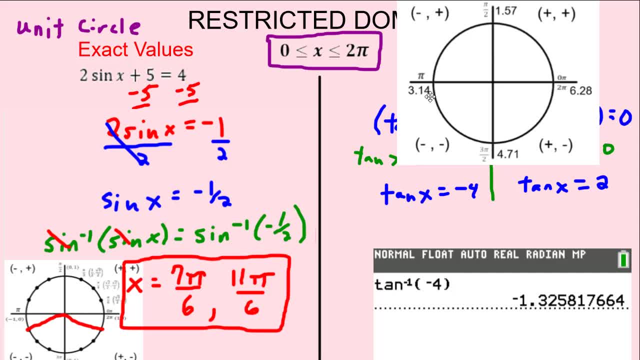 this little handy dandy guy here where I just kind of put the decimal equivalent. so pi is 3.14, half pi is 1.57, just so I know what I'm talking about. because, remember, the calculator is only going to give you tangent in the first or fourth. 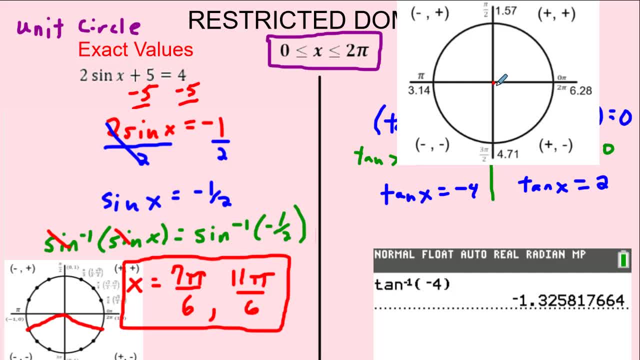 quadrant. in this case it gave us fourth quadrant because that's where tangent is negative. so it's something like this: negative 1.32, like that. but where else is tangent negative? where else are the signs different? aha up here, so the calculator won't tell you the other version of that, where. 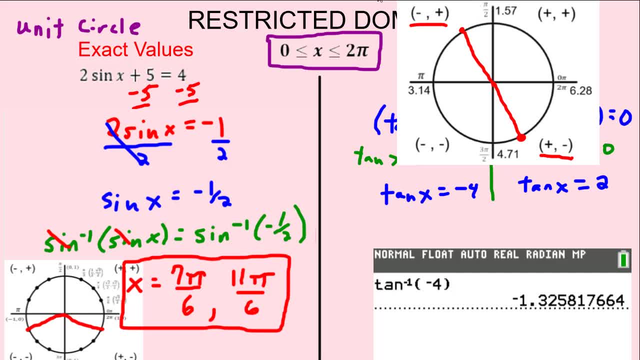 tangent is negative. so you have to be careful. you actually have to find these bad boys, so let's go ahead and find these. I'm going to kind of clean up my notation here. so in the calculator I did what inverse tangent. so another way to write, that is, we could have said: 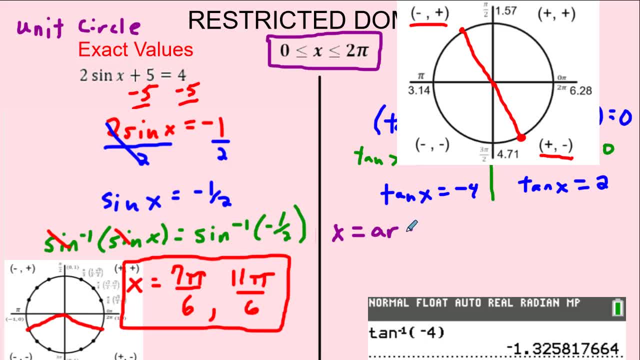 tangent. so I want you to be familiar with this. X is what X is: the arctan of negative 4, so you may see this notation like a multiple choice question or something like that. so that's really what I found. and what did I get? I got negative 1 point. I'm just going to truncate again: negative 1.325. I'm just going to cut off at three decimals. now be careful: is that in my restricted domain? it's not in the restricted domain. that's a huge bummer. so I got a. 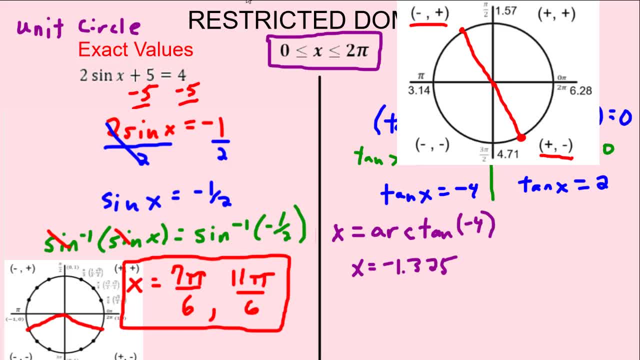 put it in the restricted domain. So let me get rid of that, So I can't call it negative. So instead of calling this negative, from here to here, negative 1.328,. what can I do? Just add two pi to that bad boy. So we're just going to add two pi to this, So make sure we're in a good spot, right? 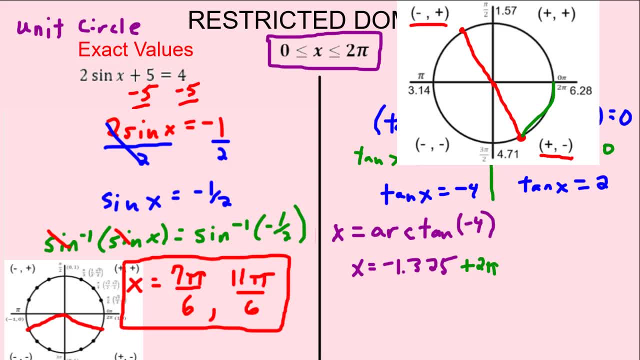 here. So let's put that in the calculator, because I want to have that exact decimal. So let's just add two pi to this and see what we come up with, And we're going to get 4.957.. Excellent, So that. 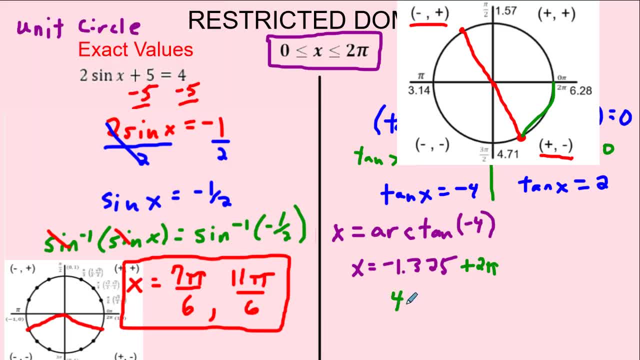 is now. it's in the restricted domain: 4.957.. Awesome, So there's one answer. Now there's more answers. So I have this: negative 1.325.. I added two pi to get back to here, but I also need this. 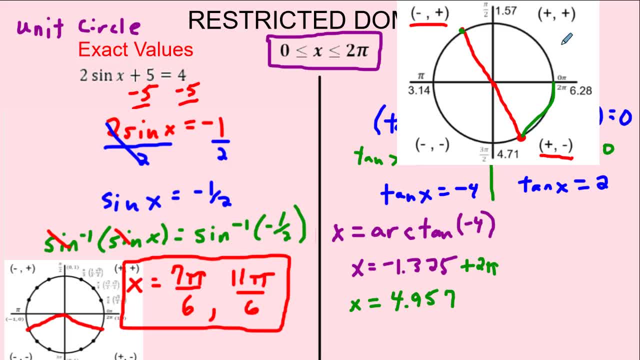 one over here. So what do I really need to do? I got to go back and I got to add a pi to get over here. It's on the other side, like 180 degrees away. So we got to go back to that negative 1.325. 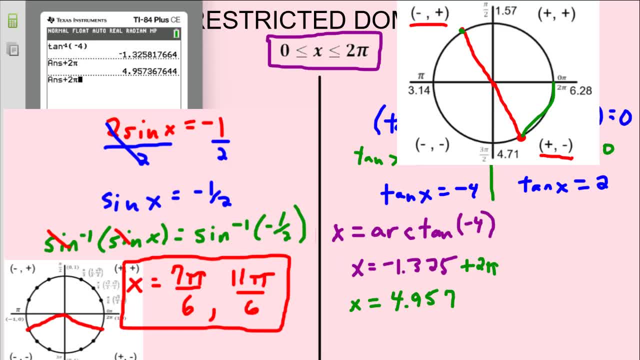 again. I'm going to bring up the exact value again. I'm going to kind of bring up that inverse tangent of negative. So I have it. And then another answer would be is if I just add a pi to it? So what am I finding? 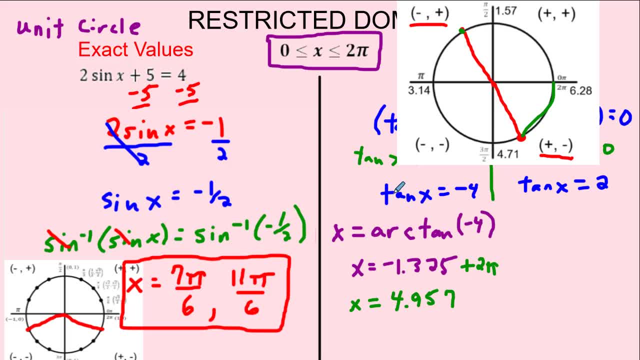 here I've got 1.815.. So 1.815.. So that's another possible answer. And what is that? That's, if I go this way, 1.815.. Fantastic. So two answers there. We got to get them both. Oh man, now we got to do. 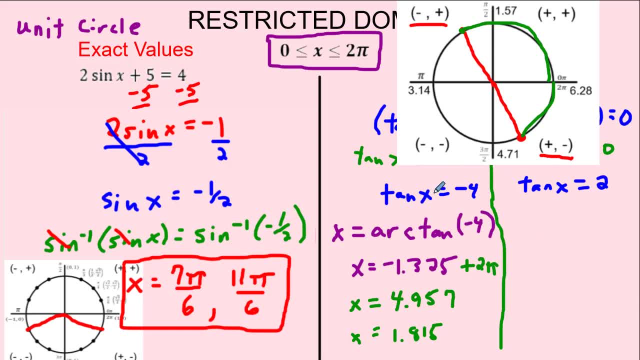 the other side, Holy cow. So what's going on over here? So we've got the negative four. Well, it could also be with tangents too. So we've got the negative four. So we've got the negative four. So again, just so we're cool with notation, I'm going to take the inverse tangent of both sides. 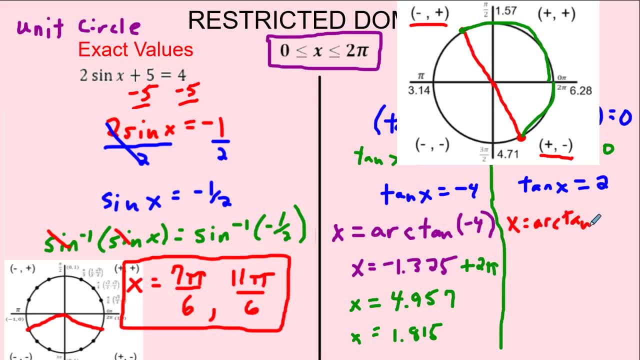 or I'm going to take the arc tan of both sides, And now I'm taking the arc tangent of two. So that's just what I'm showing when I'm typing in the calculator. Now, what's the calculator going to give me? Well, I know tangent's going to be a positive two. It's going to give me something in. 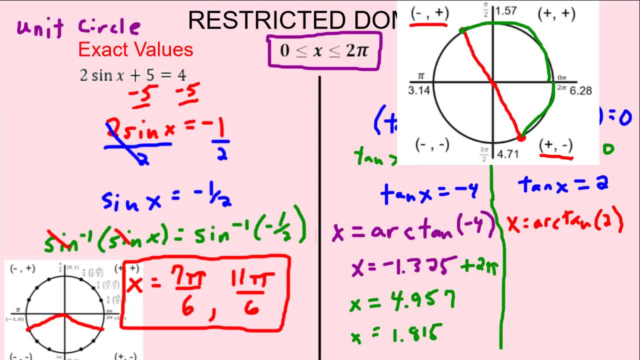 this first quadrant. So let's find that bad boy. See what we got here. Ah, where's it at. There he is. Let's clear this out. We got a lot going on over here, So let's do inverse tangent of two. 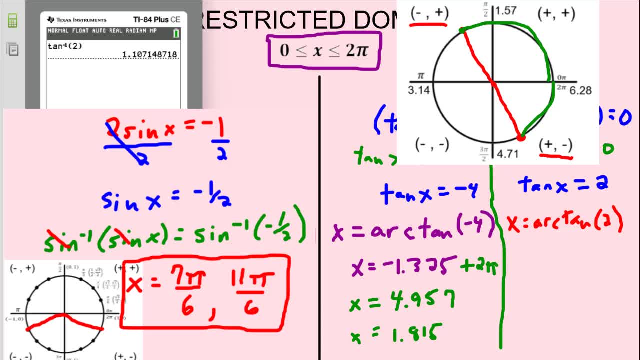 Inverse tangent of two And we get up with something like this: 1.107.. And that's in that first quadrant. there, So 1.107.. Let me write that down before I forget it. We've got 1.107.. And again, roughly it's not 1.57.. 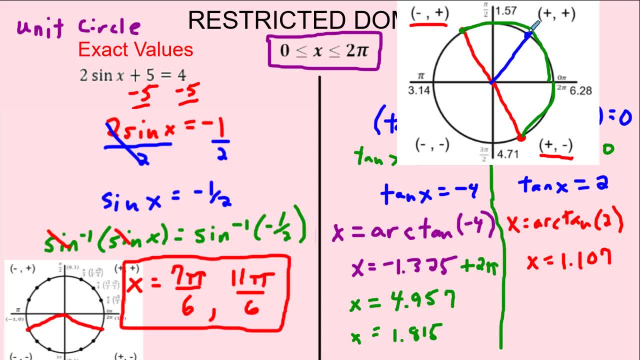 It's something I'll do. this one in blue, It's maybe something like this. Just a rough estimate. Really, I'm just worried about the quadrant. So this little chunk here, 1.107.. Where else is tangent positive, though, Because it's not going to be both. 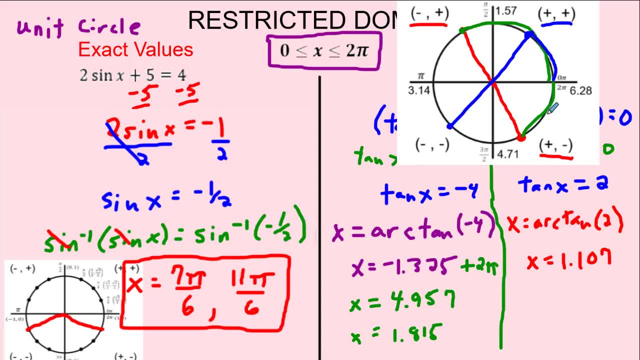 It's straight across. I love tangent. It's just straight across. So luckily this one's in my restricted domain. All I got to do to add to this one is what? Just add pi to it. I just need to get to the other side. Ah, let's try that again. Add pi to that bad boy. So we can just take that answer. 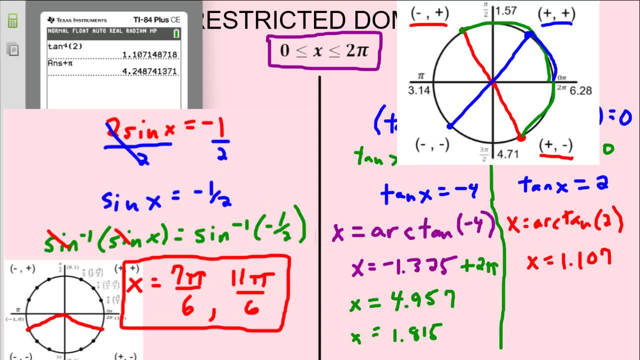 add some pi to it And we are going to get to 4.248.. Ah, let me write all that down: 4.428.. Fantastic, There, it is right. there, Boom. So what are my answers? So I've got these that are in the restricted domain. 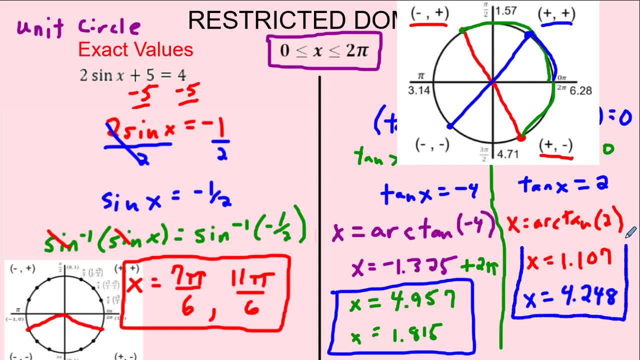 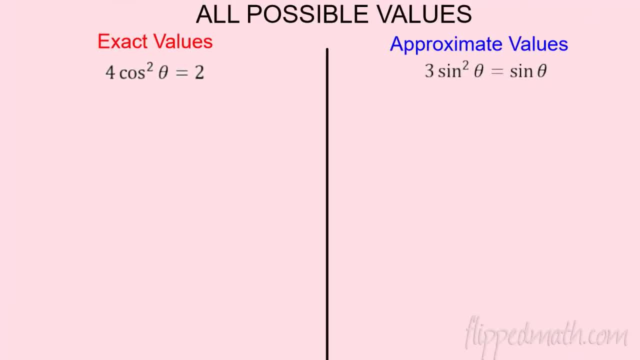 I've got these two that are in restricted domain, So I've got four possible answers between 0 and 2 pi that all work. That is awesome. Okay, Let's do it. when we don't restrict the domain, Let's go ahead and knock them out if I want every possible sine value or cosine value or tan value that can. 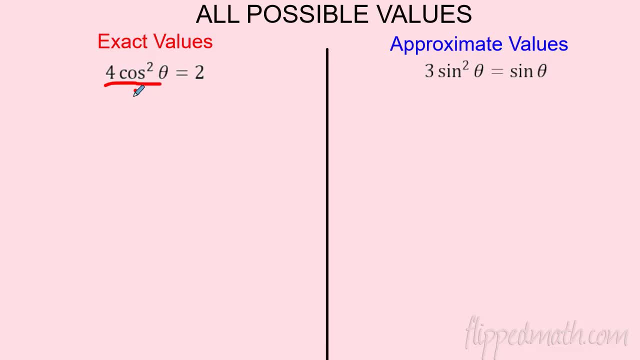 do it. So can I solve this equation? Sure, Just knock it out like you're solving an equation. I want to get, in this case, theta. You can use x if you want, or theta, The standard, for the same thing. I'm going to use theta just for some reps. That cancels that out. 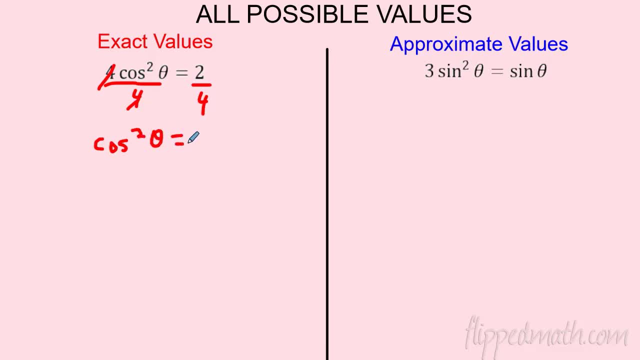 And I'm looking at cosine. squared theta equals. I'm going to write that as one half. Ooh, that's nice, because I'm looking for exact values. And again I'm going to. how do I get rid of that square? though? I actually have to square root both sides, So I'm going to square. 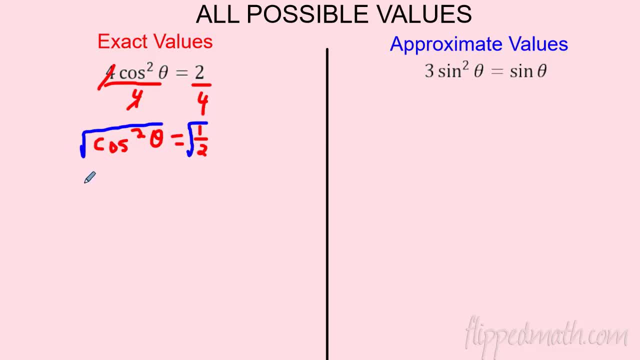 root both sides Very interesting. Well, that's cool because cosine squared, square rooted, is just cosine. Now, be careful. when you introduce a square root, what happens? It becomes plus or minus a square root. Now, what are you allowed to do with square roots? 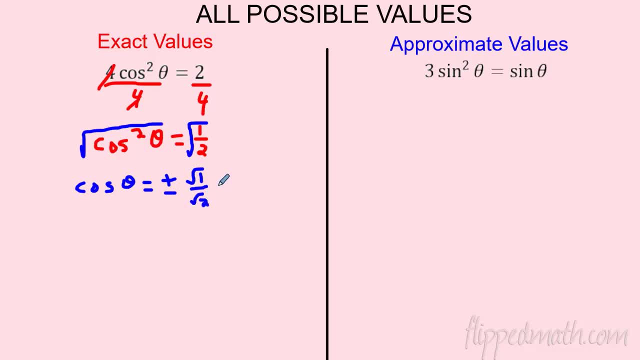 You're allowed to square root the top over the square root of the bottom. And then, what is the square root of one? It's just one. What's the square root of two? Well, it's the square root of two, But you got to rationalize the denominator, So we've got to go ahead and times this by radical two. 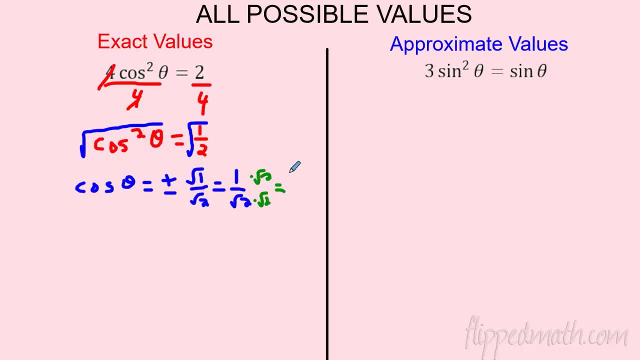 times this by radical two. Well, this is intense. So on top, to get rid of the denominator on bottom, it looks like I'm looking at radical two. Square root of two times square root of two is two, and don't forget that is all plus or minus. Let me just read the whole problem. So in the next couple of weeks, 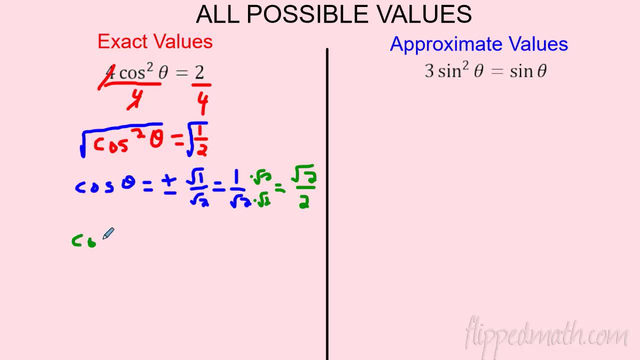 or minus. let me just rewrite that bad boy here. so we have it. so i'm looking for. the cosine of theta equals the plus or minus square root of two over two. so bust out your unit circle here. just draw a little rough sketch here. and i'm looking for where does cosine do this? well, i know it's going. 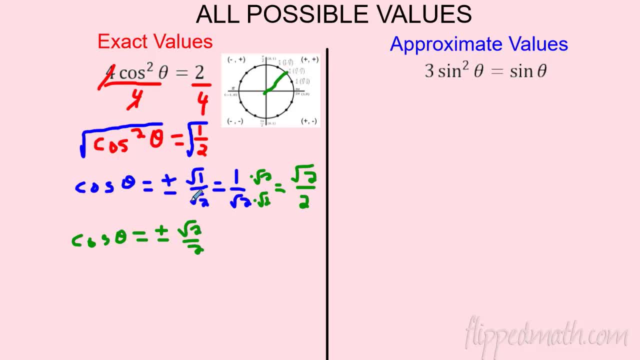 to happen at pi over four. that's the classic radical two over two. and since i'm talking about all the plus ones, uh, for cosine, that's here and here's where it's positive. what about for negative? radical two over two? that takes care of this one and this one. it's all of these holy cow. so there's. 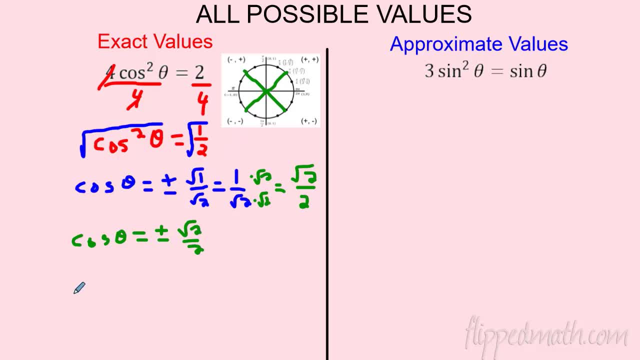 a bunch of them. so how do i write all this out? well, there's a couple different ways. you can just take the initial one you got. so we're gonna, i'm gonna write it two ways, if that's coolio to start. so the first one is: yeah, it was pi over four, and then it could be: um, what from pi over four? 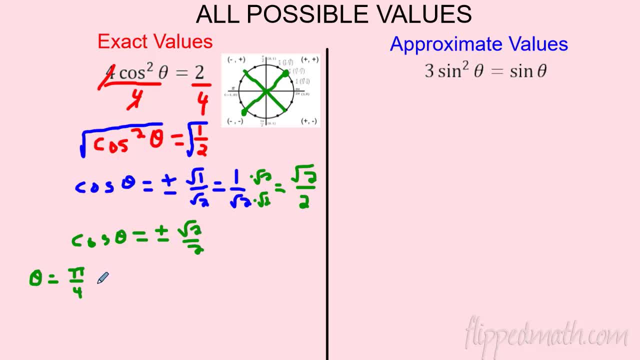 it could be what pi later you could say: plus pi n. ah, this is a very interesting one, or i could have said: what was the other one i got over here for the negative. i got um, what is that? three pi over four and it happens what it happens every pi over and from there. so like adding: uh i. 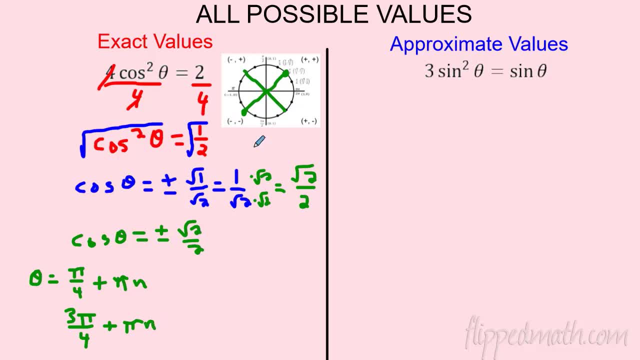 always think of degrees back. pi is 180. it's just the other side of the line. so this is all possible angles. you could just list all four individually if you wanted to. i guess that would be kind of tedious, but you could list pi over four, three, pi over four, five, pi over four, seven, pi over four. 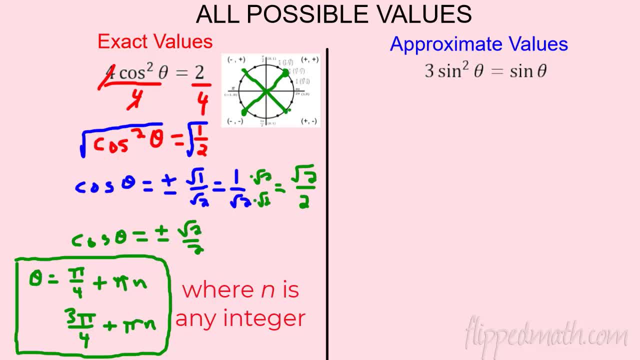 and just save two pi n. and again, the key to this: this is where n is in integer. for that awesome, that is every possible value. we gotta add that little uh caveat there. okay, can we do it for approximating? yes, we can. let's do it right here. sound like bob the builder there? yes, we can. um. 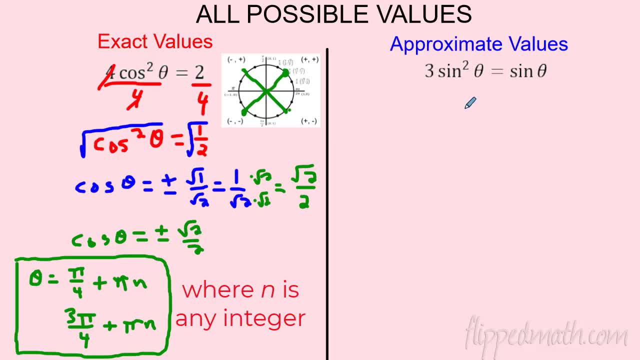 be careful here. don't write this down again. i'm big on. don't write this down. this is what a lot of people like to do. they like to just divide by sine on both sides. this is not good. don't do this. so yes, it works okay. 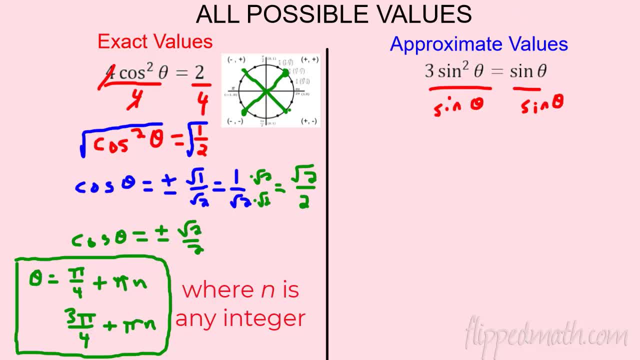 you want the answers, but it's going to cancel out some answers. so anytime you can't really divide by that variable like that, that's going to cause problems. so what are you going to do then? well, we're actually going to set it equal to zero. this is a factoring problem, so this is a classic one. 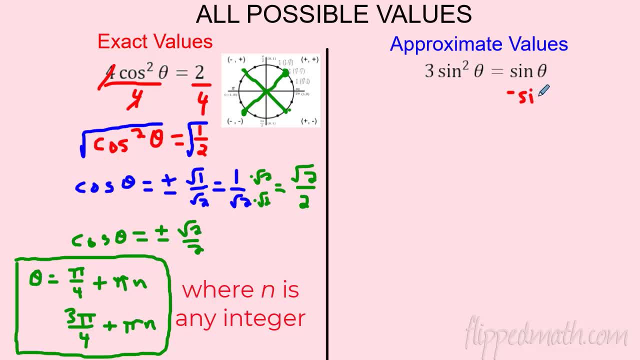 you're definitely going to see this. uh, so we're going to subtract sine from both sides, sine of theta. if you truly dislike theta, you can write x, you can rewrite them. it's the same thing, but we are talking about an angle, so it's not too bad to write it like that. so we're looking at what this 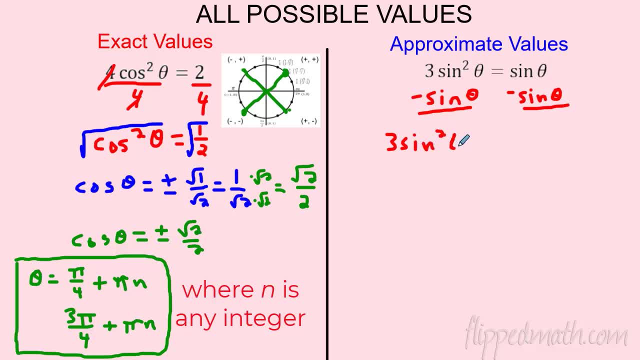 is three sine theta, minus sine theta, and what's that going to equal? there's nothing on the right side, it's going to equal zero. so now, maybe you can see it. now it's a factoring problem. what is the greatest common factor, or what do they? 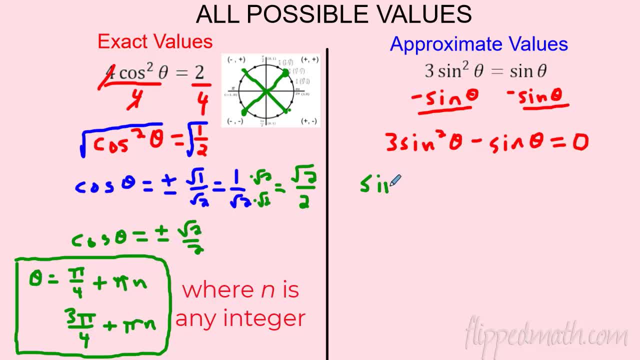 share. they both have a sign. so i'm going to take a sine out and there's a sine. and what's left? well, i've still got a three. it was sine squared becomes sine, so it's three sine, and then i took the sine out, so this will just be minus one. awesome, now we need to solve this bad boy. so i always think of it. 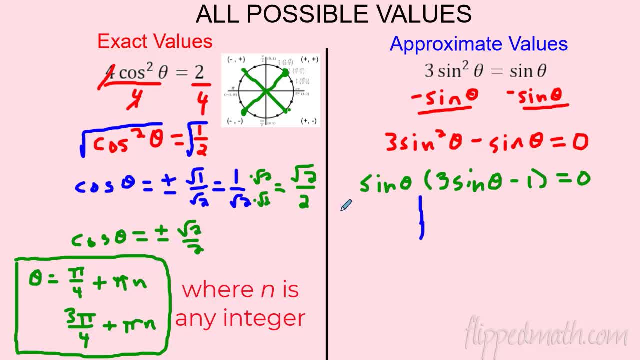 separate problems. What makes this zero over here? So we're thinking about: hey, when does the sine of theta equals zero? Also, we got to think about this- parentheses right here: When does three sine theta minus one equals zero? And then we got to find all possible values. where it happens, I love. 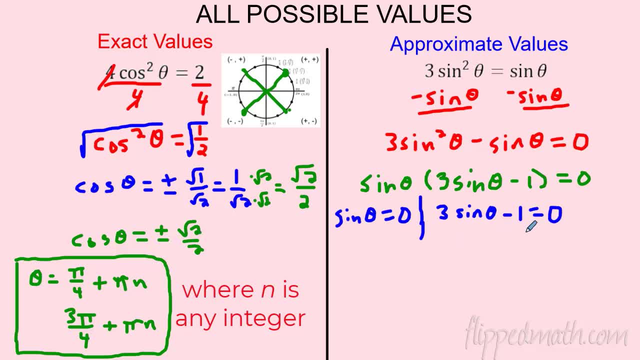 it. This is intense, So let's solve this real quick. I can add one to both sides and divide by three, So I'm going to kind of skip some steps there. I hope that's cool. Add the one, you get one, divide by three. We're really looking for when does the sine equal one third? Okay, so I 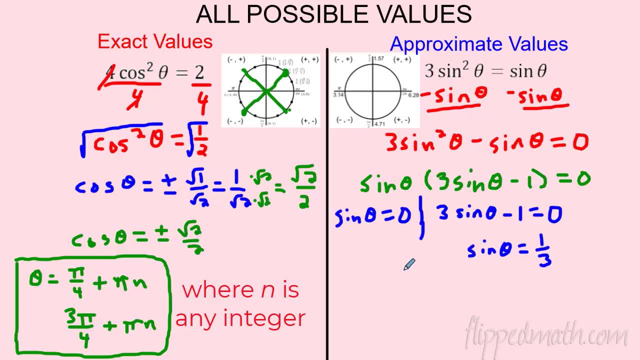 popped up the approximate, just a little rough circle so I can see, So I can go to my calculator and say: or I don't need it for this- When does the sine? I know it's approximate, but when does the sine equals zero? Well, I know sine equals zero, here at zero, And it also equals it over here. 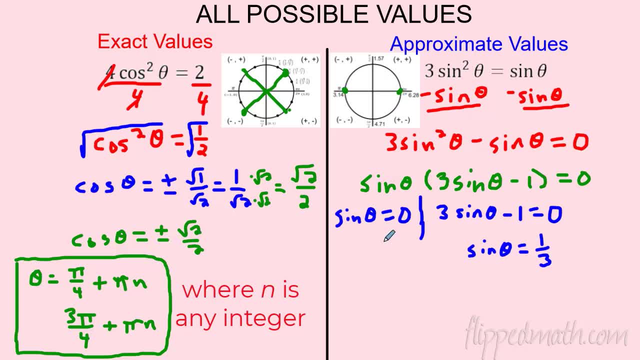 at pi and then back here again. So I know this is going to make an answer at zero or pi. I'm just going to say pi And then don't forget, if it happens every single time, what am I adding back and forth? You're? 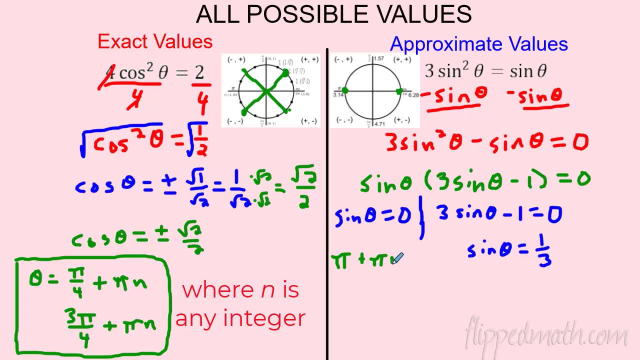 adding plus pi n. So I'm taking care. that's going to take care of the quadrantials here, the ones right across this. It's going to take care of that. Awesome, How about over here? So what makes one third? Now I definitely need my calculator, So I'm going to go to my calculator, pop that up. 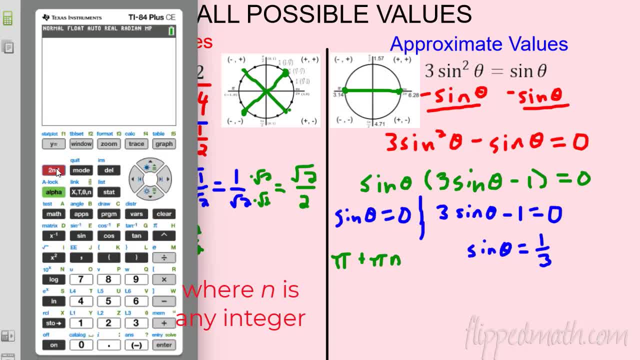 It's going to let me clear all this out. There's a lot going on here. I'm going to say, okay, what is the inverse sine of one third? So I want that angle And it's 0.339 if you truncate, So it's going to be 0.339.. 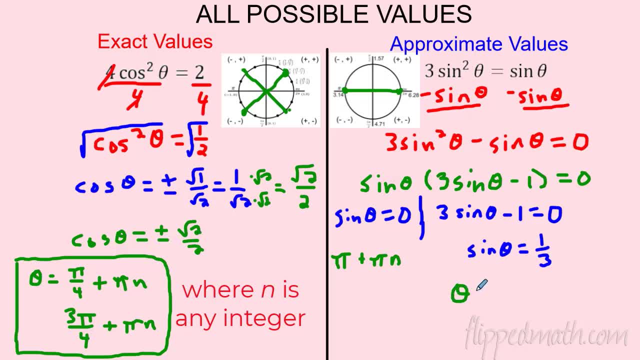 So I know that's going to say, hey, one angle for theta is 0.339.. Boom, there it is. But I know, because it's an inverse trig for sine, it's only going to give it to me one and four. So it gave me this one right here. That's it. It didn't give me the. 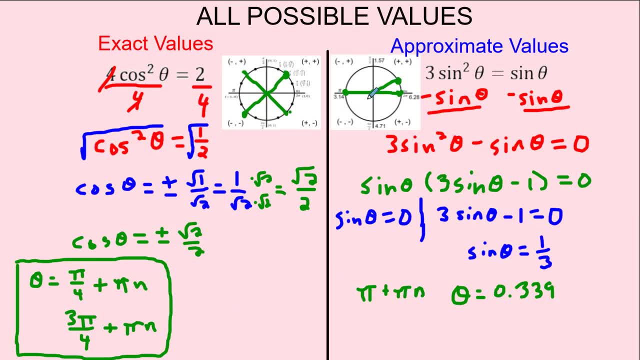 other one. So where else is sine positive? So if sine is positive here, sine is also positive in the second quadrant. So I'm going to go to my calculator and I'm going to go to my calculator, so I'm looking for this bad boy over here. So if we're talking about this, angle here is 0.339 above. 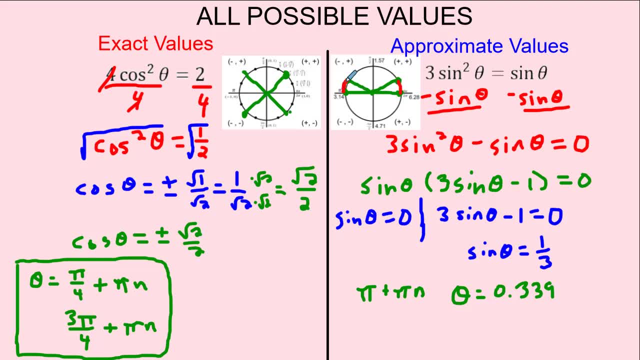 the x-axis here. then I need to find a guy who's just a little bit short of pi. He didn't quite make it to pi, So he's 0.339 below pi. So back to the calculator. Holy cow, here we go. So I'm. 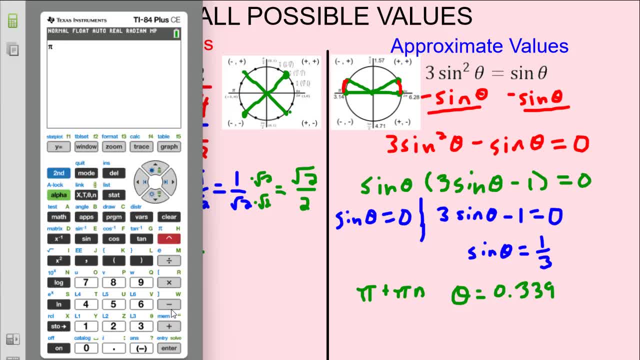 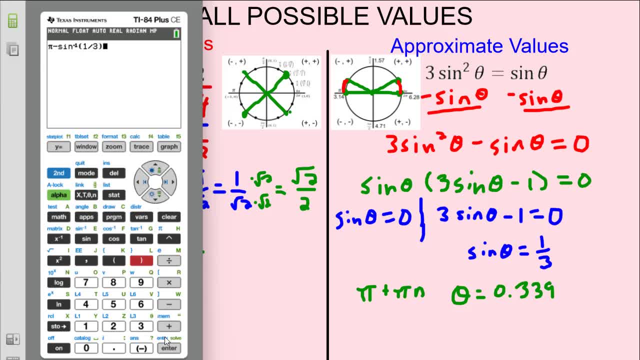 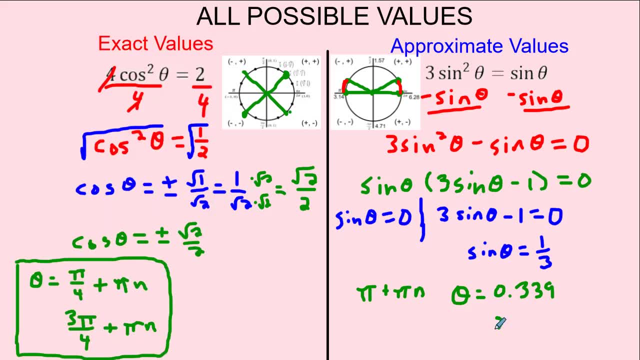 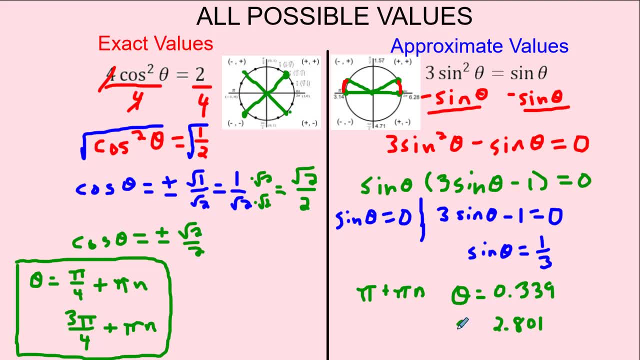 the 7. I'm just going to truncate it here. So here are my two possible angles here. Holy cow, But now, because it's all approximate values, forever it keeps repeating. So I have to do what to these bad boys. I have to add 2 pi to each of these because I'm going to go around the circle. 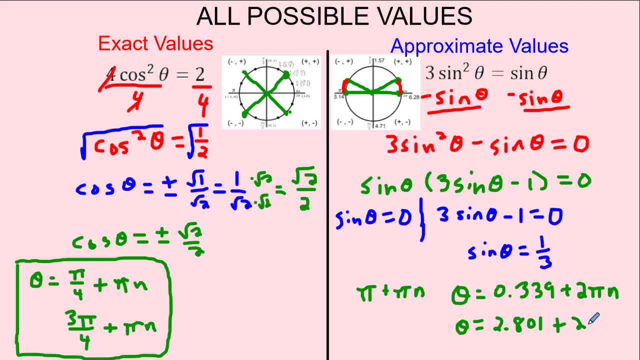 forever and ever, And I'm going to do this right here And I'm good to go. Don't forget, theta can also equal this bad boy over here, And that takes care of all possible solutions for this. Wow, Just to double check. if 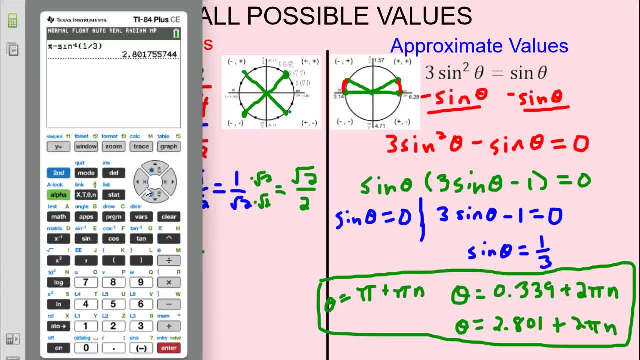 you want, you can actually graph these bad boys in the calculator. So this is kind of a nice little trick for checking if you just graph them. So I can graph: y equals sine squared. Just be careful how you type sine in, So you're actually squaring the entire equation. So you're actually squaring. 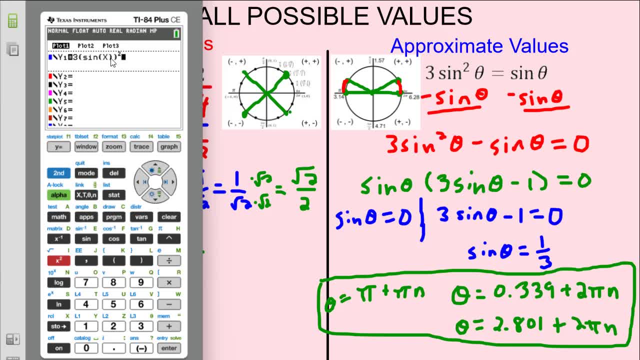 the entire sine thing. So check how I wrote that I took sine of x, put in parentheses, squared the whole thing. So I want to know: when does sine squared x equals sine x? Sine x sounds like cold medicine or something. And then I'm going to graph these bad boys. Make sure you zoom trig, so you 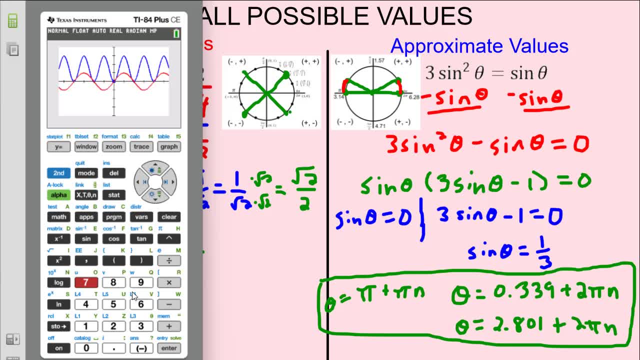 have a nice window And I know I'm going quick here because this is just a quick check. But the ideal is: where are these hitting? They should be hitting at every pi plus pi n. So let's just check it, So trace pi, And what does it give me? You can see they hit every pi plus pi n. So I'm going to 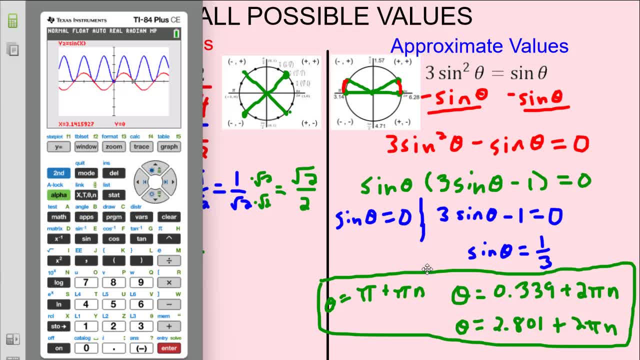 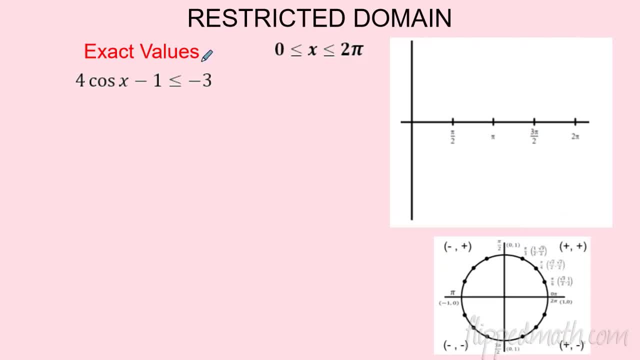 get perfectly here. That's where they cross. And again, if I type these in the exact values, that's all the places they cross. That's super cool, Awesome. All right, We only have six problems to do. We've knocked out four of them. All right, Let's solve this bad boy. So, just like our. 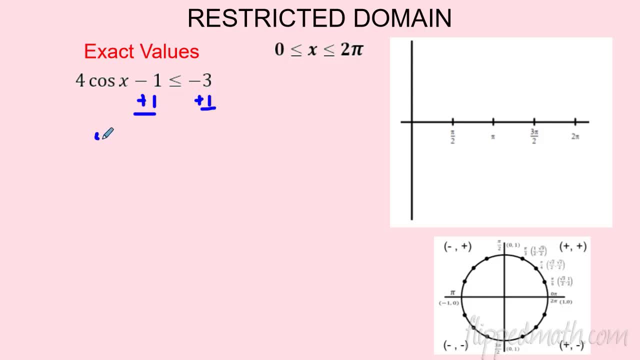 equations. we're going to go through our steps of trying to get x by itself. So if I want to get x by itself, got to add one to both sides. So I'm going to add the one to both sides And I'm looking. 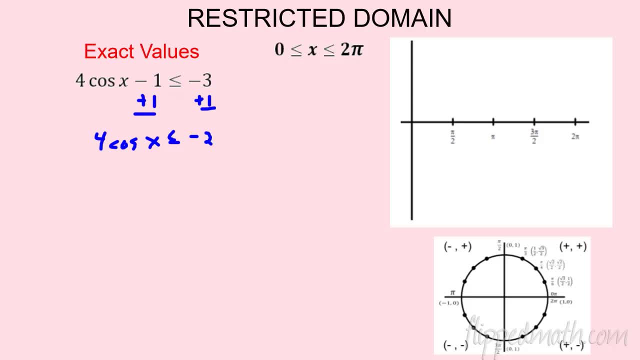 at what It's less than or equal to negative two. Then I need to get rid of that four in front. So I'm going to divide both sides by four. Divide both sides by four And we're looking at: cosine x is less than or equal to. I'm going to go ahead and reduce that negative one half. 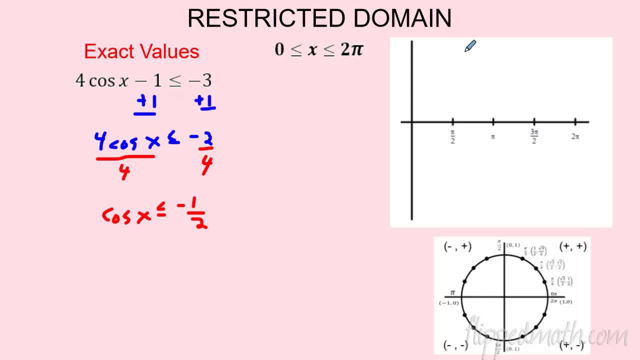 Awesome. Now notice: this is less than. So what I want you to do is include a little sketch- There's some rules we can memorize, but let's just kind of almost like test values- of where this answer is true. Okay, So I know I want less than, but let's find the. let's just find what x is going. 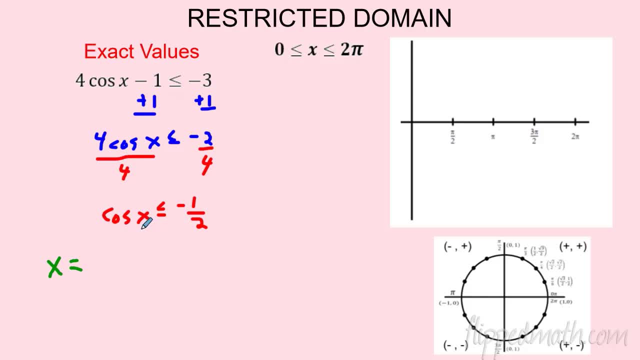 to be here where it's equal to part of this. So where does cosine x give you a negative one? So we're going to do the inverse cosine negative one. Here's the unit circle. We've got that restricted domain again, So I'm going to look at the inverse cosine negative one. So I'm going to look at the. 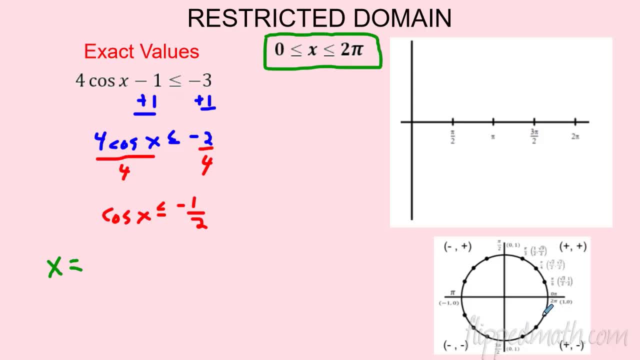 between zero and two pi. Don't worry about that whole n thing. And where is? do I get negative one half for cosine? It looks like I'm going to get it right up here at this bad boy up there. So what is that? Two pi over three, Awesome. Is there another place that's going to happen? Yes, So 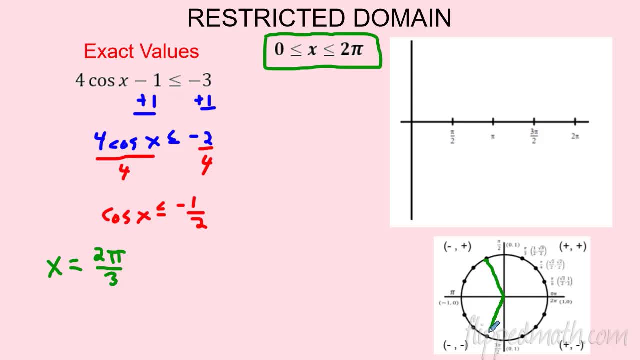 I know it happens up here. Cosine is also negative in this quadrant. So if I add another pi over three past that, I've also get four pi over three. So here are my point of interest. So the question is, is it happening in between these two or on the other side of it? Like are my? 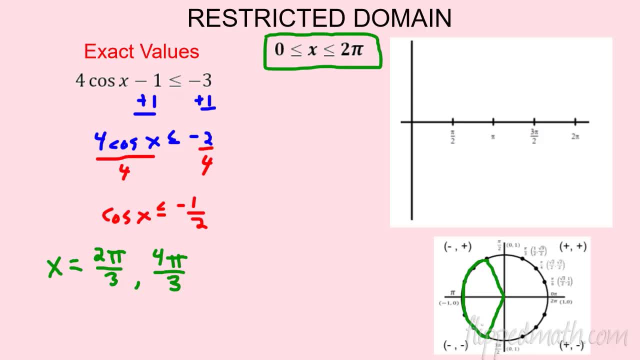 answers in here or on the outside of this. So to do that, let's make a little rough sketch here. So let's just graph this first part right here. Let's go back to this And I want to graph this side of the equation like: y equals four cosine x minus one. So it can be rough, I just want to. 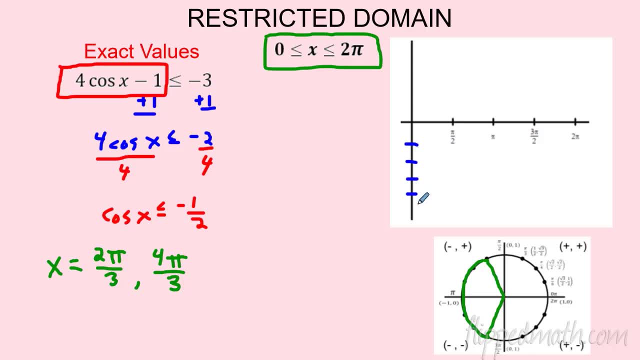 get an idea. So let's go one, two, three, four, five, And I know that it's got this. um, it's new axis. So I'm going to go one, two, three, four, five, And I know that it's got this. 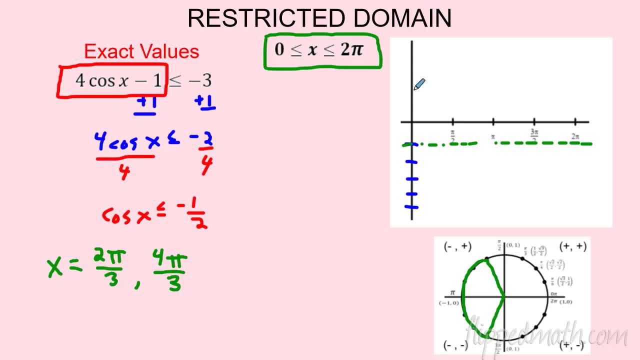 right here at negative one. I know it's cosine, So it's going to start above one. Oops, I should use the same color here. I didn't realize we're going above two. So I'm going to go four above for cosines. at one, two, three, four. It starts up here. I know cosine is two pi later I know. 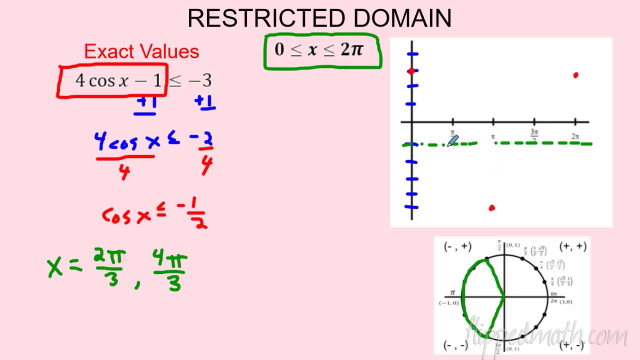 in the middle. it's going to be down here One, two, three, four- And I know you love graphing these. I think trig functions are awesome. I can do this all day long. There, it is right there, So. 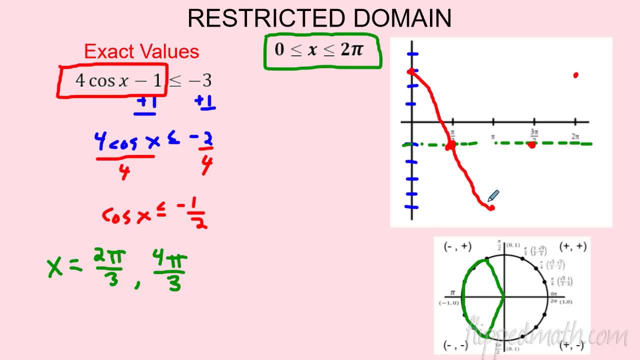 I've got this really rough idea. Oh man, It looks curvy enough. Okay, That side's got some nice curve to it. Very nice, Very nice, Uh, excellent, Now let's graph the other side. So what about this one? I want to know when is? 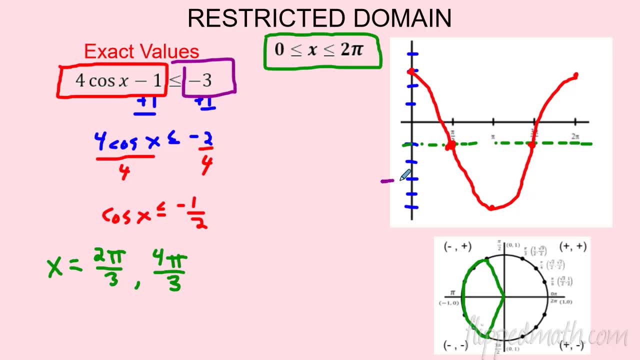 it less than or equal to negative three. So one, two, three. here's where I'm concerned about Boom, This line right here, And this is where they hit. So this is my whole: Y equals negative three, And those are the point of intersections which, if I did it right, should these: 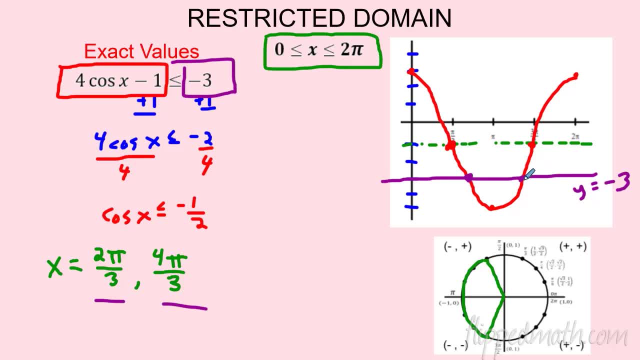 these points right here. So does that look like negative? two pi over three and four pi over three? Sure does, man, Congratulations, You nailed it. Those are the two points. So I like the highlighter because I think the highlighter is awesome. Um, I'm looking for when is the trig? 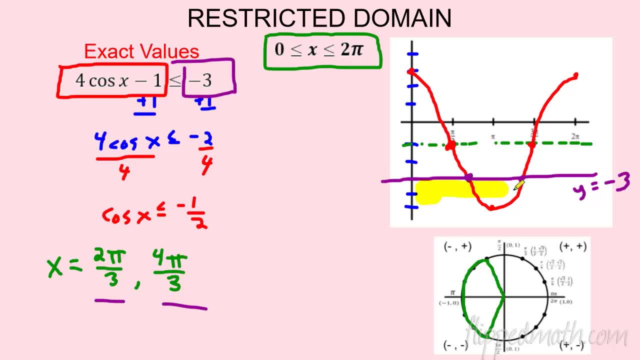 function less than negative three. So I'm actually looking for all of. I'm looking for this underneath the curve. Now you don't have to get a highlighter out, although I highly recommend it because it's really fun. Uh, and now? so where are my solution sets? They're in the highlighter. 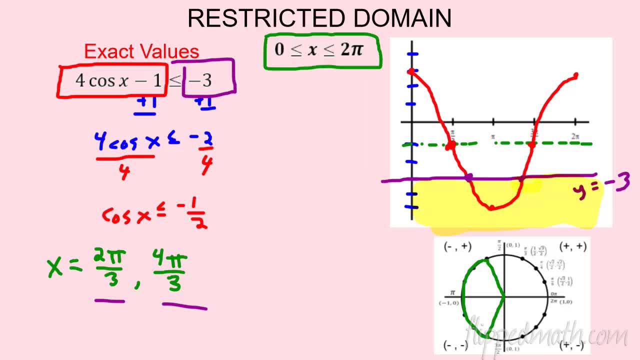 region. Let's go ahead and write those bad boys out, So I know I can see the actual answers where it goes. So I'm going to go ahead and write those bad boys out, So I know I can see the actual answers where it. 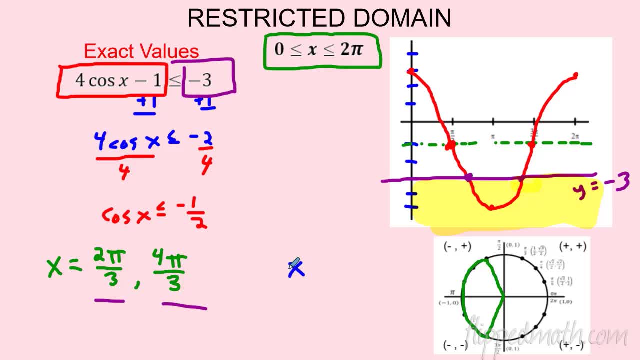 crosses. Now what does that mean? My X values are squished in between what. they're everything below the curve here. So they're below two pi over three, and I'm sorry. Yeah, And so it's. my Xs are going to be between two pi over three and four pi over three. So that is my solution, set for all. 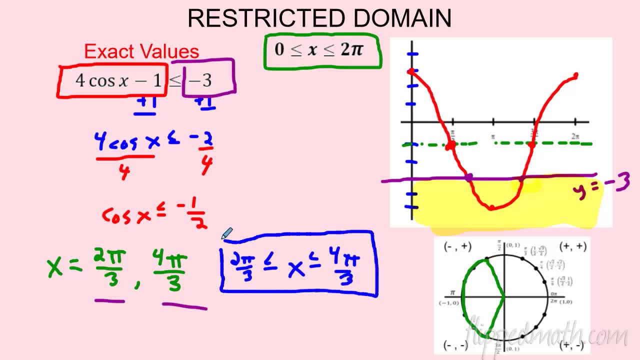 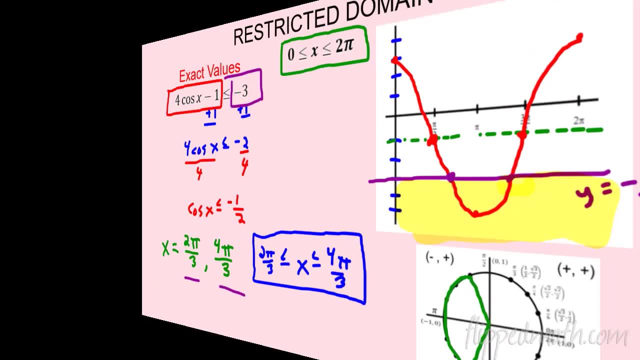 possible answers that make that equation true. So I like to have a little rough sketch: plug and chug and you're good to go. Woo, That's fun. That's a big problem. right there, We nailed it All right. The finale, This is just kind of weird. Uh, this could happen a couple of times, but uh. 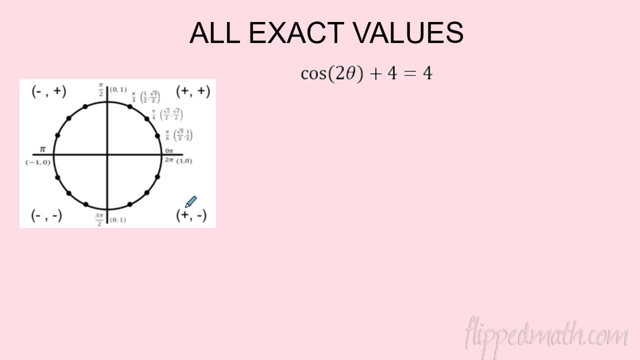 I just want you to be prepared for it. Mr Bruce never taught me that. Um, check out this. what I do. I mess with the inside here. So we've got this horizontal dilation or I'm changing the period of this, but just solve it like a normal equation. Let's not worry about that yet, Let's just go. 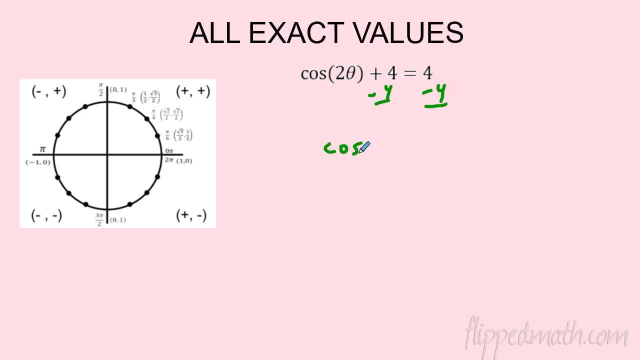 through the steps of solving this. So I'm looking at: cosine of two theta equals what? Zero? Oh, that's awesome. So now let's just figure out when this happens. So what am I really doing? So I got kind of slack. I'm not. 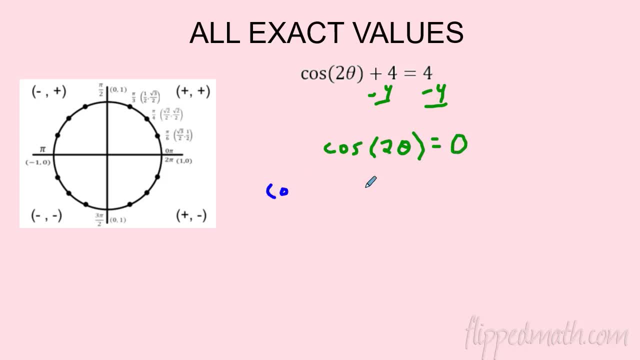 going to lie. I'm really saying, Hey, when does cosine of two theta equals zero? but I'm actually saying I got to get rid of cosine. I'm doing the inverse cosine of cosine. Now in my answer keys I did show them all So you can see all those awesome steps. but this is what I'm really doing. 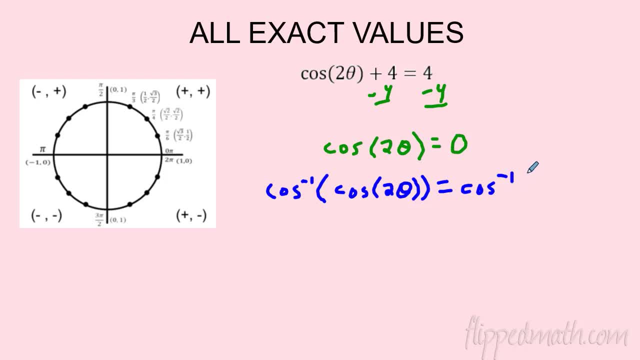 I'm actually saying: take the inverse cosine of both sides, Excellent. Now why am I doing that? Well, what happens? Well, this cancels this, So they cancel each other out. And what's left? We're left with two theta. So here: 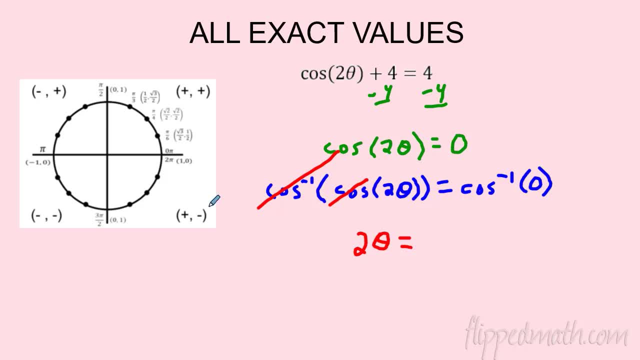 I really got to show the steps. Now, what is the inverse cosine of zero? Well, go to your chart and find where's cosine zero. It's going to happen up here at pi over two and there, So go ahead and just write it out. So I'm looking at these two points on the graph and I'm doing all exact values. 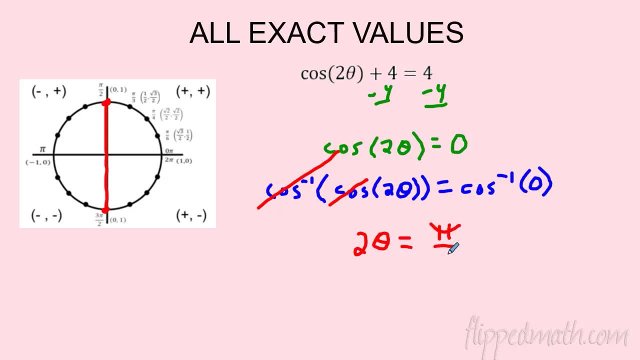 So I'm starting at pi over two. If I add pi to that, I'll be at my next one And pi n, So that'll take care of pi over two, three pi, and we keep going back and forth, adding pi and pi. 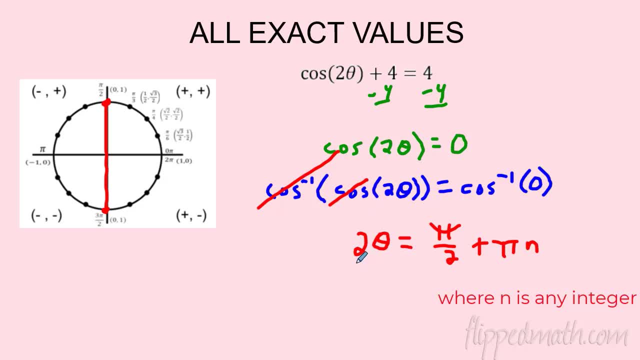 But am I done? No, not done. Why? Because that's two theta. So what do we got to do? We have to divide both sides by two. And why do I do that? That'll actually give me theta. And now, when I do this, what happens? I've got pi over two divided by two. 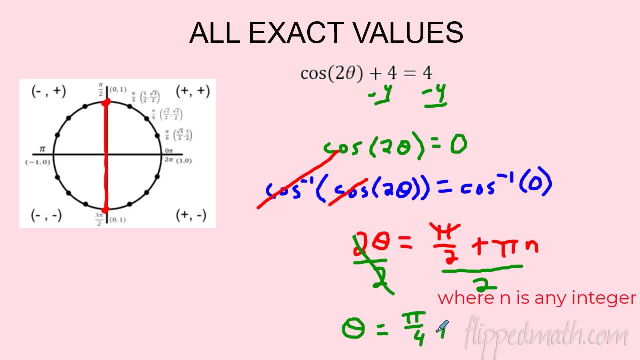 well, that becomes pi over four, plus what's pi over n. divided by two, It is pi over 2n. So it does mess up your answer And it made sense. You don't have to. So it does mess up your answer And it makes sense. You don't have to. 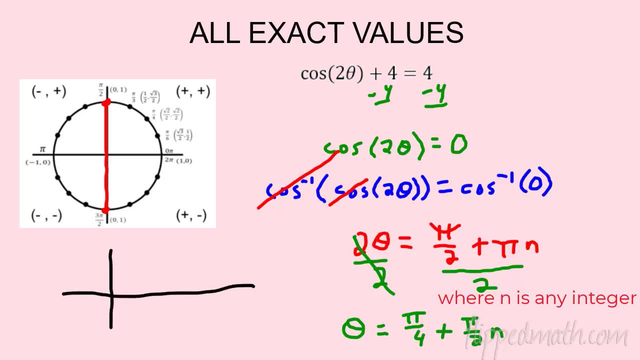 write this down. but if you think about this, if you graph that cosine, uh, up there at four, a normal, it changes the period. so you're going to get, normally you just get one set of answers. but now, because it's littler like that, if i drew in, where is it hit? so if i drew, where is it hitting at four? 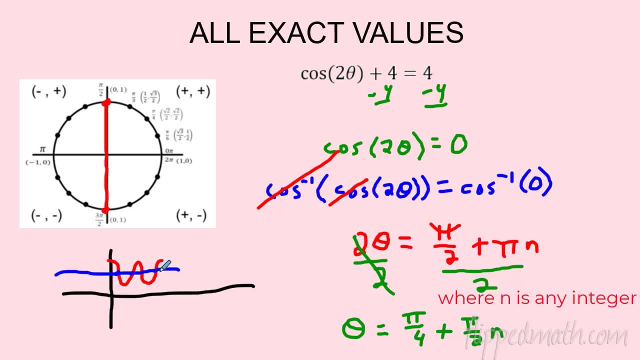 that'd be something like this: you can see there's one, two, three, four answers. uh, happening. there's more answers happening in that normal. that was in our normal two pi range. so that's why i have more answers. that's why it's going to mess things up. it's just getting more answers. okay, you can.